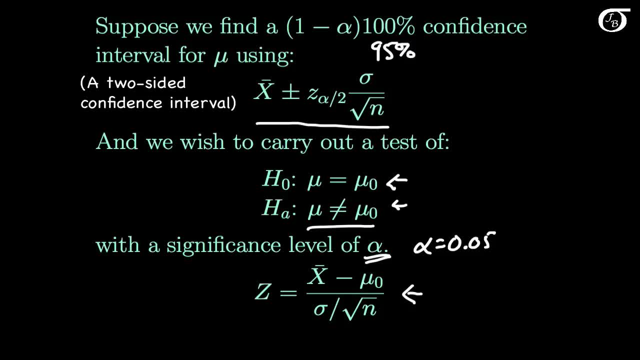 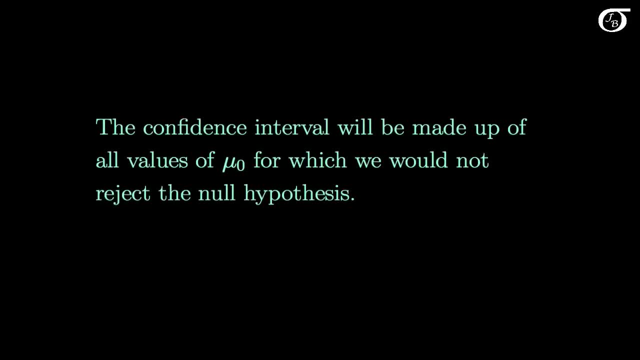 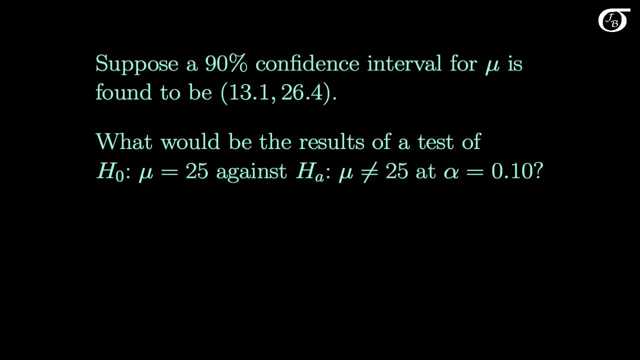 Then there is a direct relationship between hypothesis tests and confidence intervals. The confidence interval will be made up of all values of mu0, for which we would not reject the null hypothesis. Let's look at a couple of examples to illustrate. Suppose a 90% confidence interval for mu is found to be 13.1 to 26.4.. 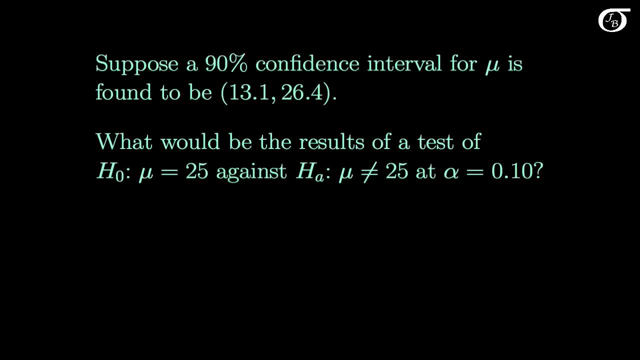 What would be the results of a test of the null hypothesis that mu is equal to 25, against a two-sided alternative at an alpha level of 0.1?? A 90% confidence interval corresponds to an alpha level of 10% or 0.10.. 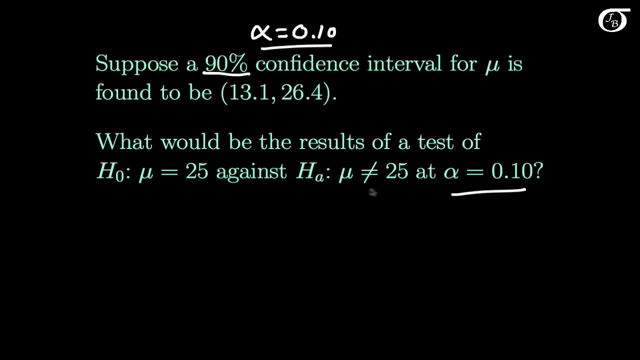 And so our two alpha levels are the same here, And the alternative hypothesis is two-sided. so there is a direct relationship between the confidence interval and the hypothesis test. The hypothesized value of 25 falls within this interval, and so we would not reject the null hypothesis at an alpha level of 0.1.. 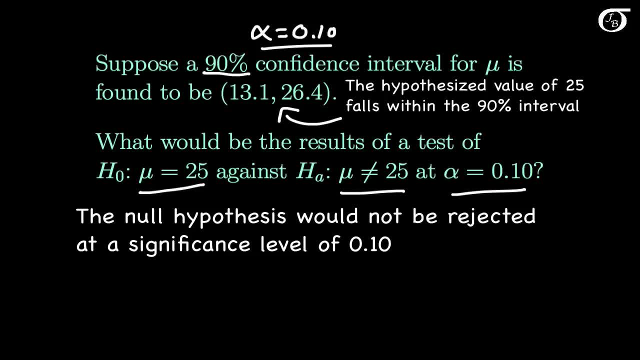 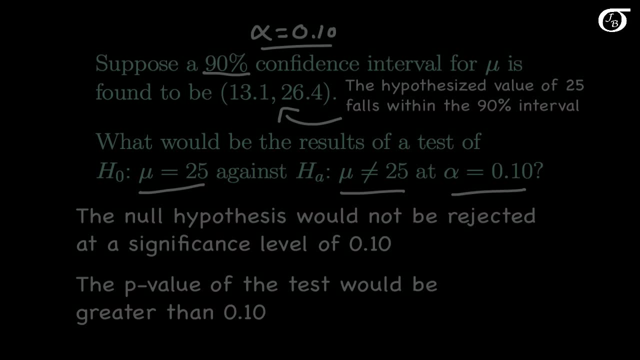 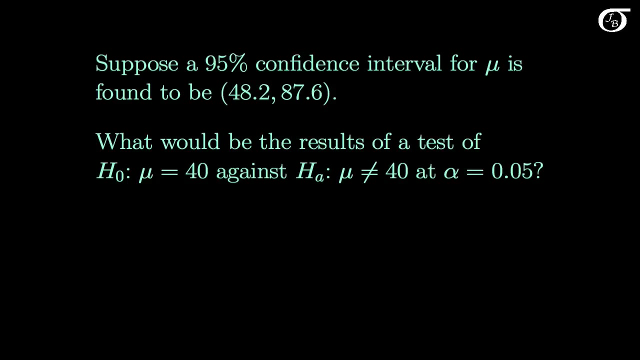 Loosely speaking, 25 is a plausible value of mu0. And since we would not reject the null hypothesis at a significance level of 0.1, we know that the p-value would be greater than 0.1.. Suppose a 95% confidence interval for mu is found to be 48.2 to 87.6.. 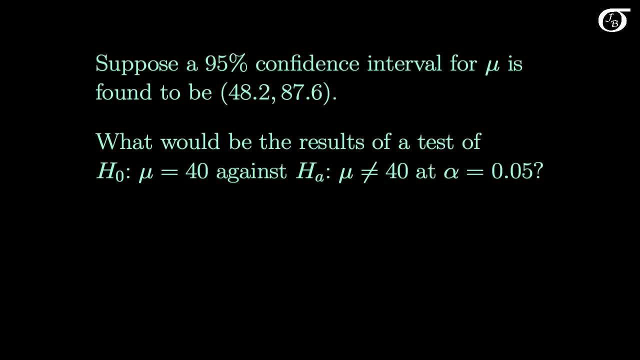 What would be the results of a test of the null hypothesis that mu is equal to 40, against a two-sided alternative at an alpha level of 0.05?? A 95% confidence interval corresponds to an alpha level of 5% or 0.05.. 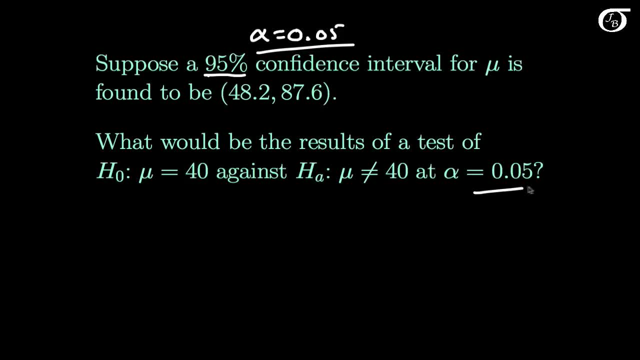 And so the alpha level for the confidence interval and the hypothesis test are the same, and the hypothesis test has a two-sided alternative, So that direct relationship between hypothesis tests and confidence intervals holds here as well. The hypothesized value of 40 falls under the null hypothesis test. 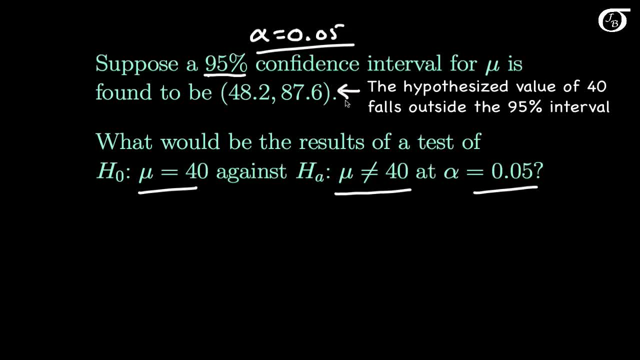 and 40 falls outside of this 95% confidence interval, And so we know that if we were to carry out the hypothesis test, we would reject the null hypothesis at an alpha level of 0.05.. Which would mean the p-value of the test is less than 0.05..